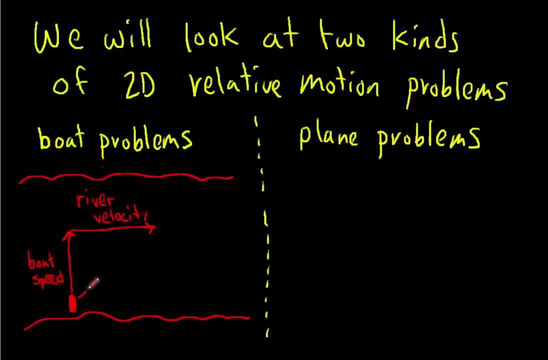 river's velocity. As a result of the combination of its speed across the river and its velocity, the boat experiences an actual route that's at an angle to where it was trying to point. In plane problems, we have much the same situation. You have a plane applying its speed in a particular. 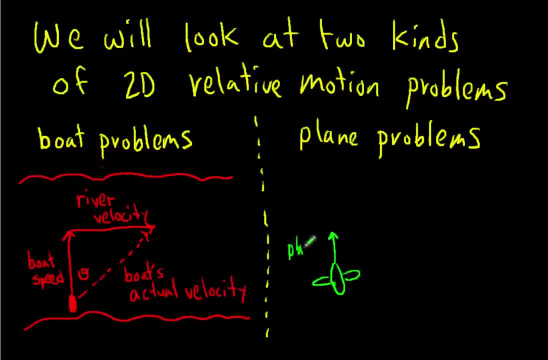 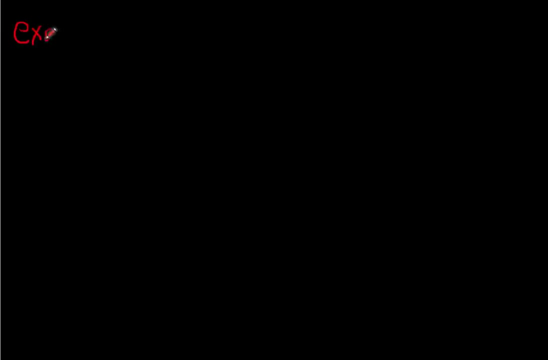 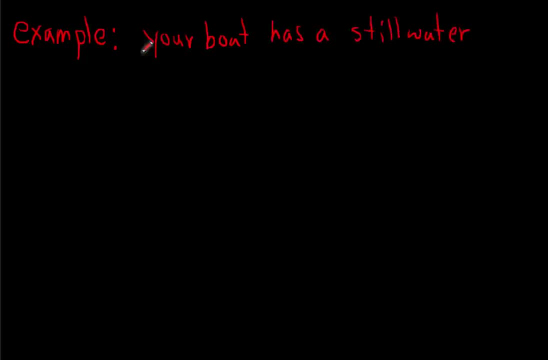 of the boat is 50 km per hour, As if the boat were flying on earth. the speed of the boat is doesn't have a speed of 20 km per hour. The speed of the boat was 50 km per hour. The speed of the boat is only 20 km per hour. And let's start with the clearly interesting. 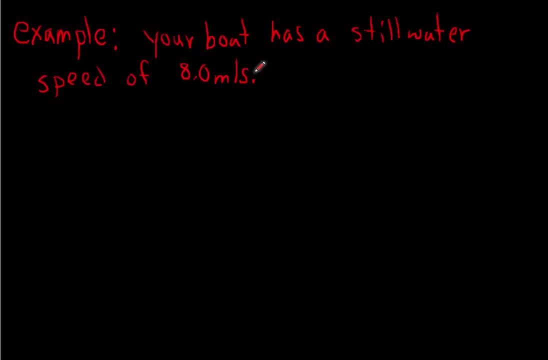 example, Explainington is not a specific rule. The way we swear in our equations brings us to the same concept. The force environment of our engine is measured by distance", w or the speed. So we got đâytoweи. It's best to draw a picture of the situation to try to understand what's going on. 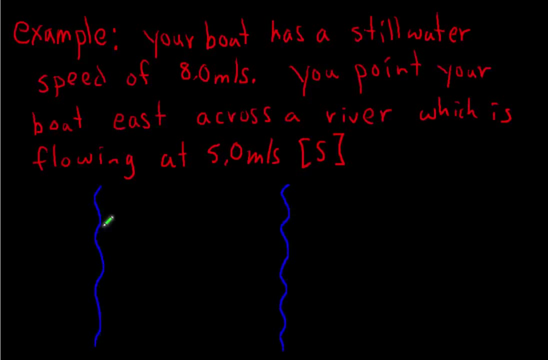 We have a river that is flowing south and you're trying to point your boat directly east, applying its speed of 8 meters per second in this eastward direction, but because the current is flowing at 5 meters per second, as a result, the boat ends up moving at an 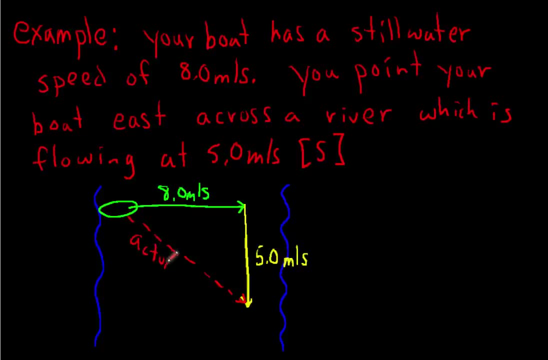 angle to where you pointed it. This is a relative velocity problem because we have two points of view. We have the point of view of the water and the point of view of the shore. We have to consider the different velocities from the different points of view. 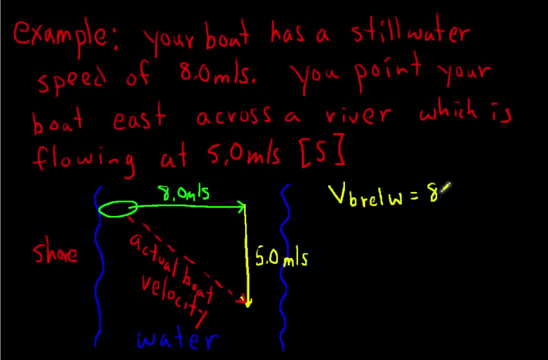 The velocity of the boat relative to the water is this- 8 meters per second- that we're applying. The velocity of the water relative to the shore is 5 meters per second, east and south. The velocity of the boat relative to the shore is its actual velocity that we're looking. 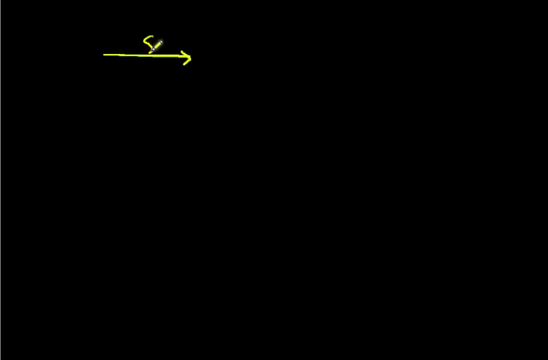 for We'll redraw this triangle so you can see how the calculation is done. It's a right angle triangle and we're looking for the hypotenuse. This is the velocity of the boat relative to the shore. This can be calculated using Pythagoras' Theorem, where 8 squared plus 5 squared square rooted. 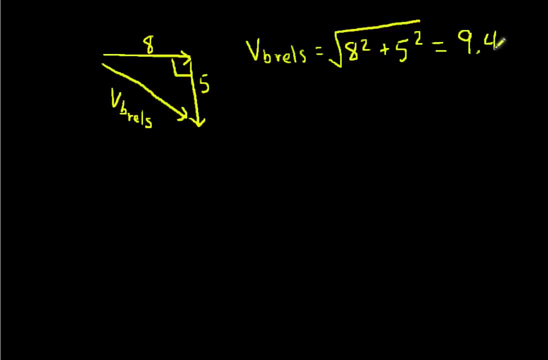 gives us the velocity of 9.3.. 4 meters per second. The angle is calculated using tan Tan negative 1 of 5 south divided by 8 east gives us 32 degrees south of east, The velocity of the boat relative to the shore, which is just another way of saying the velocity. 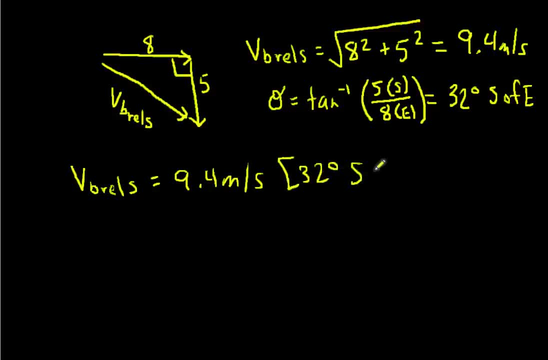 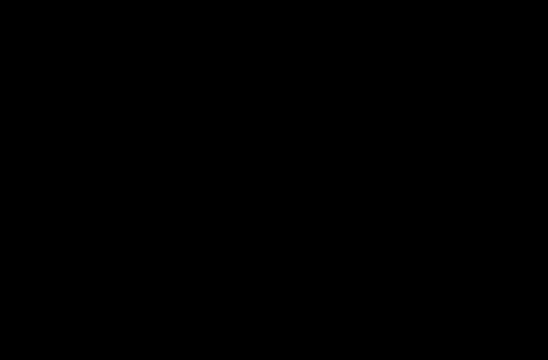 that an observer on the shore would see is the 9.4 meters per second at 32 degrees south of east. Part b of this problem asks: if the river is 25 meters wide, how long does it take the boat to cross? 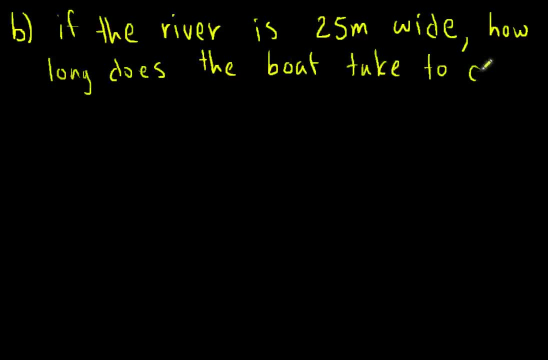 The velocity triangle we established in the first part of the problem was 8 meters per second to the east, with 5 meters per second to the south, resulting in 9.4 meters per second and an angle of 32 degrees. This is the velocity vector triangle. 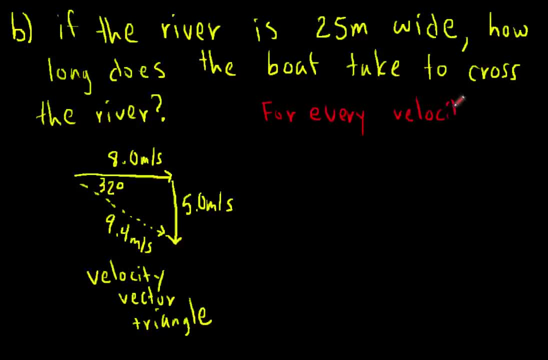 For every velocity vector triangle that we have made up of its three components, there is a corresponding displacement vector triangle with matching angles and sides. We don't know all the sides of the displacement triangle, but we do know directly across the river is 25 meters. 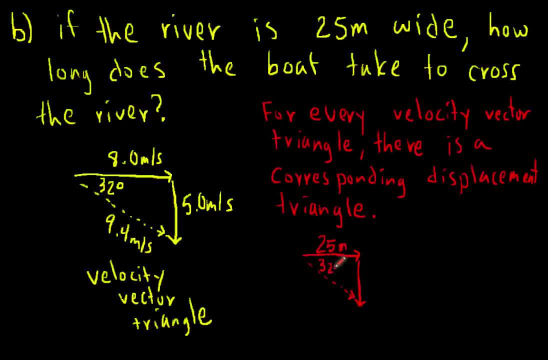 And we do know that it has a matching angle to our velocity triangle of 32 degrees. So we can use the formula: v equals d over t, because we're talking about constant velocity here on matching sides of the two triangles. So for example, the two horizontal sides are matching sides. 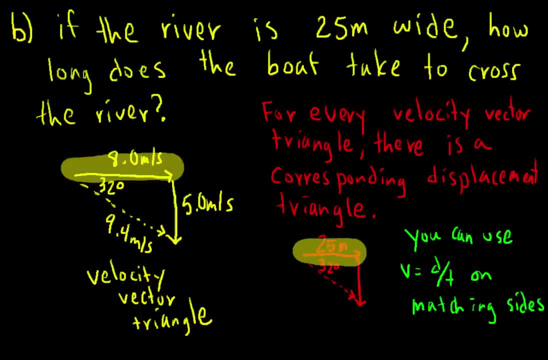 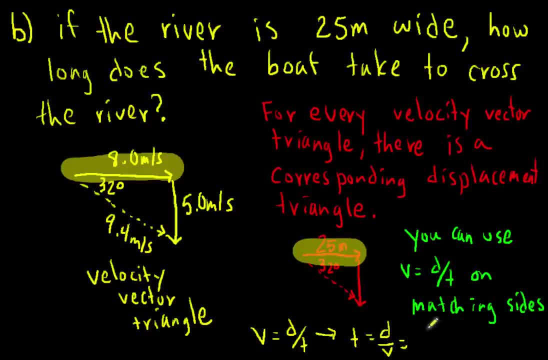 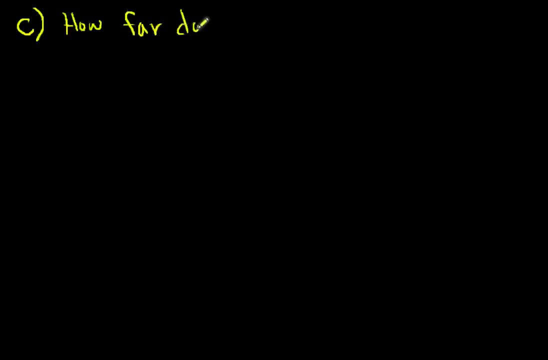 In part c. we're going to ask: how far downstream do you end up? In part c? we're going to ask: how far downstream do you end up In part c? we're going to ask: how far downstream do you end up? 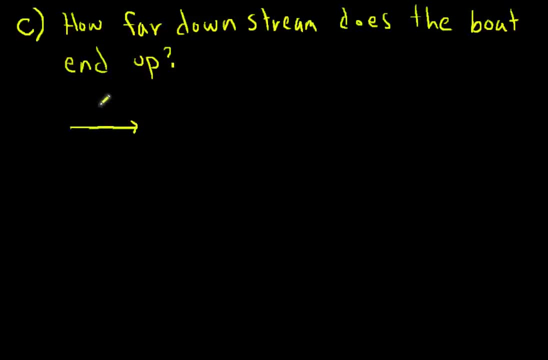 And again we look at our matching triangles. The velocity triangle is 8 meters per second to the east, with 5 meters per second to the south, combining to make 9.4 meters per second. at 32 degrees, The corresponding displacement triangle is 25 meters across. 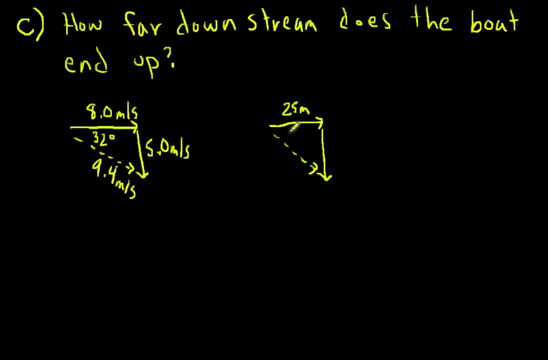 at an angle of 32 degrees And we're looking for how far down you end up or the distance in the y direction. Now these are our two matching sides: the 5 meters second and the dy, But to solve this we need a third piece, we need time. It's important to realize that. 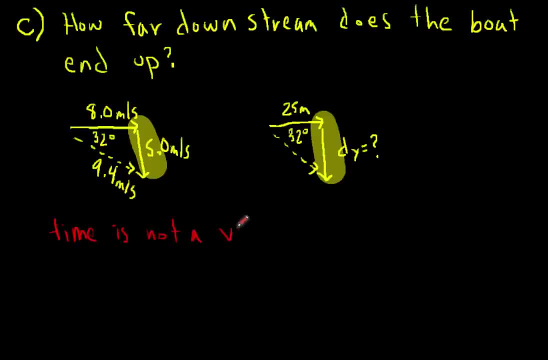 time is not a vector. Time doesn't care about direction or which way you're going. As a result, the same time can be applied to all sides of the triangles. So the 8 meters per second takes 3.1 seconds, The 5 meters per second takes 3.1 seconds And 9.4 meters per second takes 3.1 seconds. 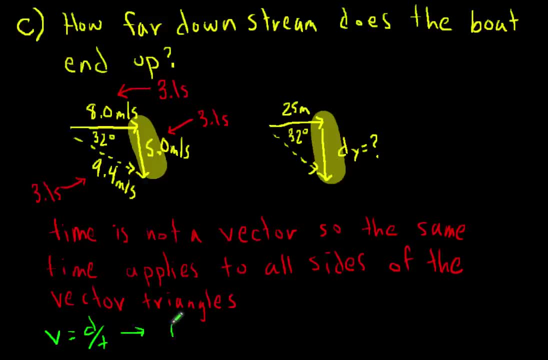 So if you find the time on one side, you can use it on all the other sides, Since v equals d over t, d equals v times t, And this is 5 meters per second times 3.125, which is the unrounded version of our time, which gives us 16 meters. 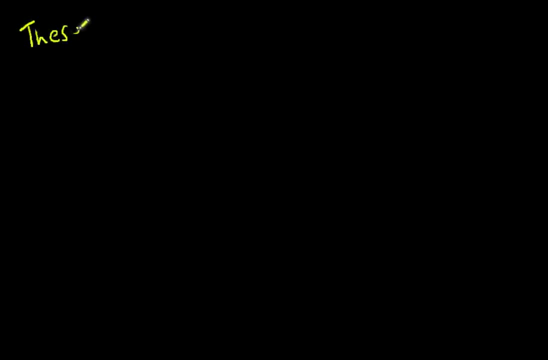 So the distance down from the triangle is 16 meters. So the distance down from the triangle is 16 meters. So the distance downstream you end up is 16 meters. These boat or plane problems come in two forms. The last form we looked at is the easier form. 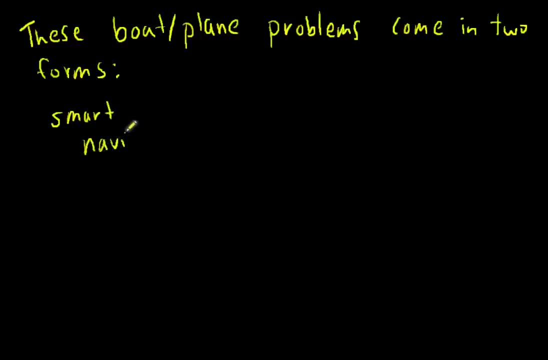 But there is another way we can look at it. I call these two problems the smart navigator and the dumb navigator. What it really just means is the dumb navigator is like in our previous example. They don't realize the current is going to push them down, So they have a river with a current. 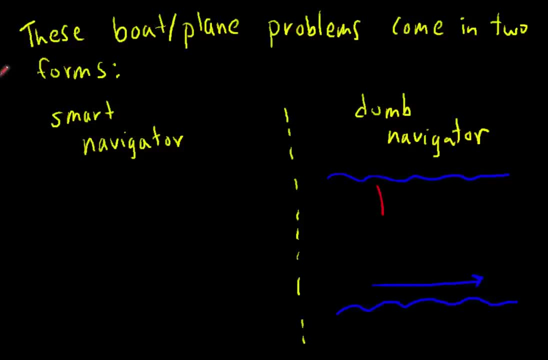 And they still try to point their boat directly across the river. And even though their point is going to be closer to the river, they still don't realize. And even though they're pointing directly across the river, because of the current, they end up at an angle from where they intended to go. 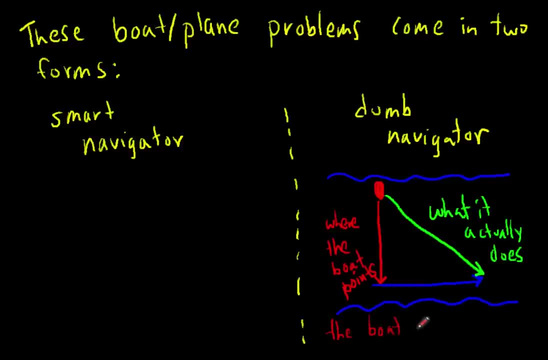 So, from the point of view of the shore, the boat ends up downstream from where it intended to be. The smart navigator knows that there's a current and, as a result, points their boat to try to defeat the current. So they see the current and they decide: if I want to end up across, I'm going to point. 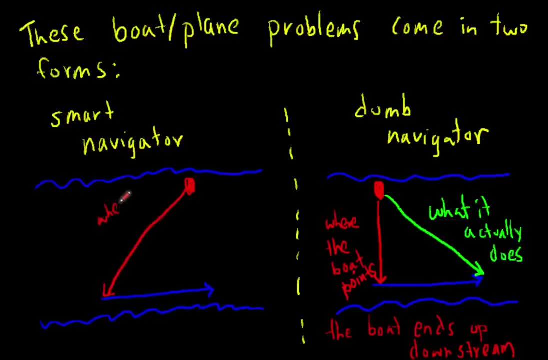 my boat at an angle to that current to try to beat it. So they point their boat at an angle And, as a result, their actual motion is the same. The ocean ends up traveling straight across And the boat ends up directly across the river. 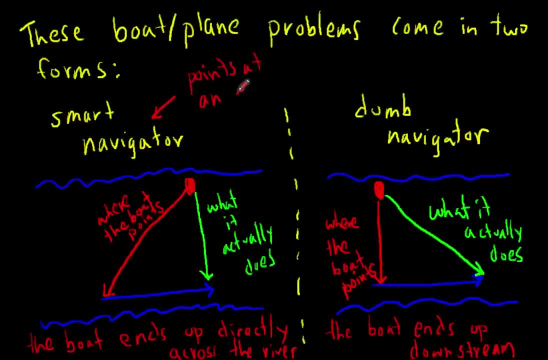 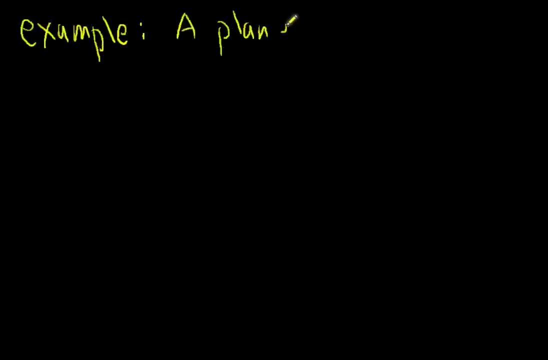 The smart navigator points at an angle to get across. The dumb navigator doesn't think to point at an angle and instead points across and ends up downstream. Here's another example, And for this example we'll look at a plane problem. 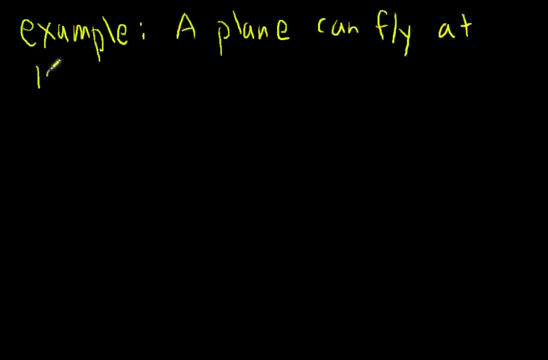 We have a plane that can fly at 100 meters per second. in still air, The plane encounters a wind that is traveling 40 meters per second to the north. At what angle should the pilot point so that the plane ends up directly west? 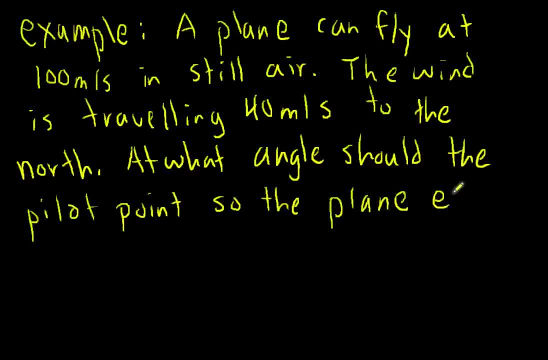 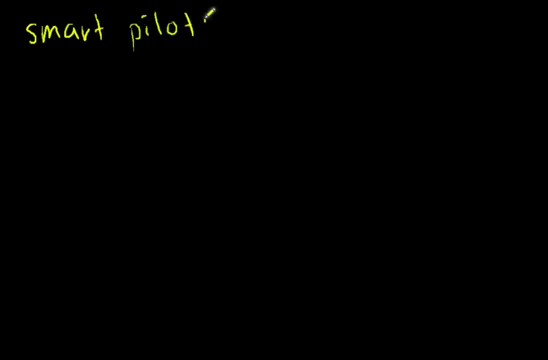 Now this pilot is a smart pilot. The pilot knows that the plane has to be pointed so that the plane counteracts the northward wind or defeat the north wind and end up to the west. 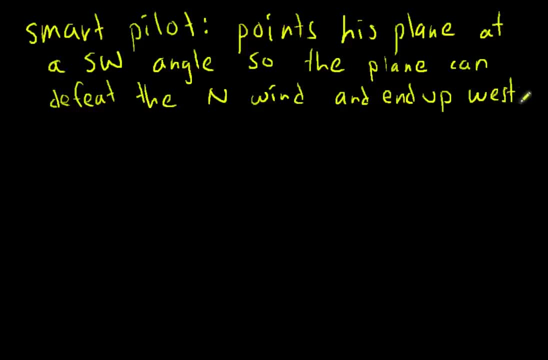 So in examining the northward wind of 40 meters per second, the pilot points their plane at a southwest angle with their 100 meters per second. As a result, the plane ends up traveling directly to the west. We say the velocity of the plane relative to the air is 100 meters per second. 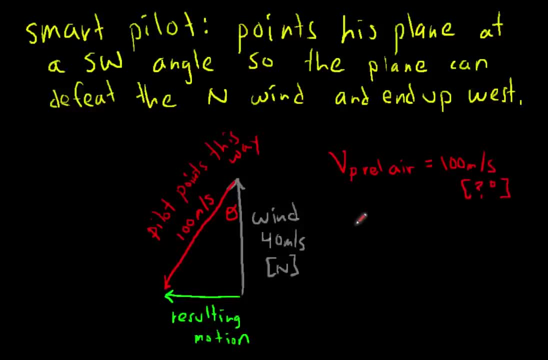 This is the velocity of the plane from the point of view of the air, and we want to know its angle. The velocity of the wind relative to the ground is 40 meters per second. This is the velocity of the wind from the point of view of somebody standing still on the ground. 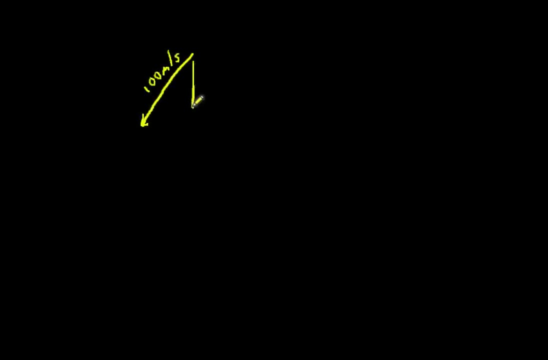 Here's the vector triangle for this problem. 100 meters per second is at an angle. 40 meters per second is one of the sides and we're looking for this angle. The 100 meters per second represents the hypotenuse of this triangle.